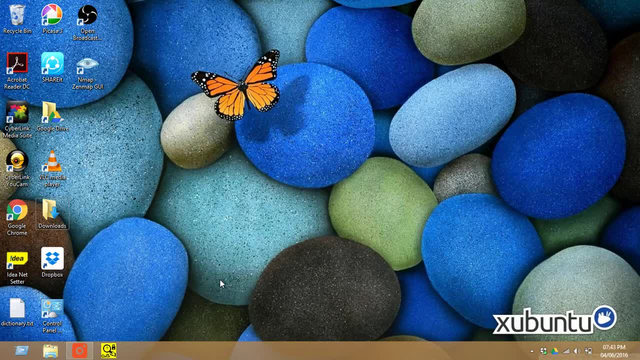 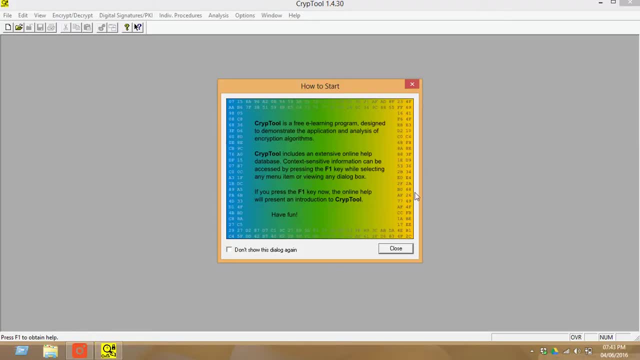 Hello viewers, in this video I will be talking about the software called as Cryptool. Now, this is software that is the Cryptool. Now, Cryptool is used for creating the digital signatures and it is an open source and free software for Windows. It is used for the crypt analysis as well as for doing the cryptography. So this is the window of Cryptool, that is 1.4.30.. So let's get started. This is the sample, that is the text on which we are going to be using. 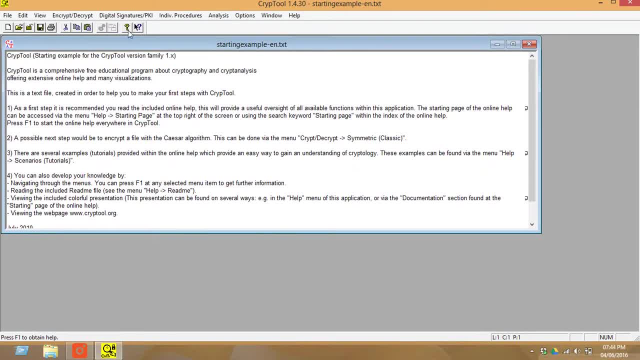 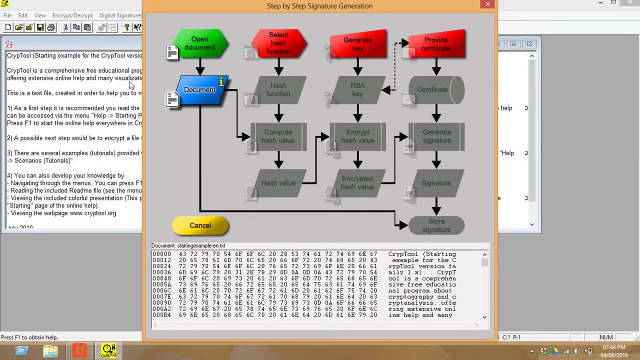 We are going to create the digital signature. So first of all, click on this. digital signatures or PKI. that is the public key infrastructure. Click on this, Go to signature demonstration and this flowchart. you can see- and this is the sample text that is shown in the background. First of all, you have to select the hash function. Click on this and select MD5 or any other as per your choice, and click OK. 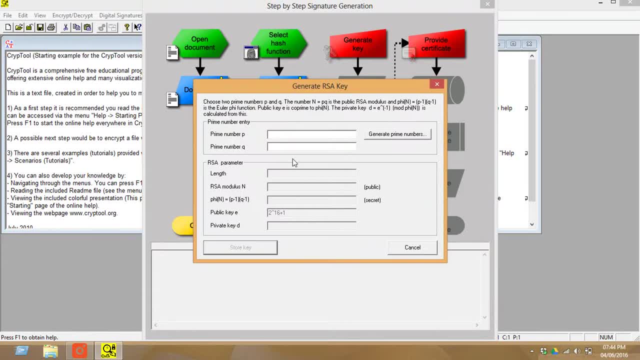 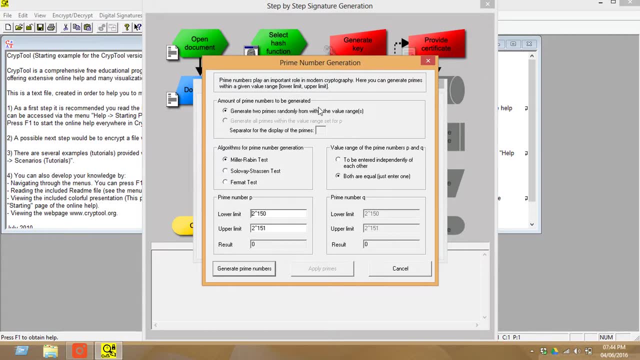 Now you have to generate the key For this. you have to click on generate prime numbers. Now make sure that the amount of prime numbers to be generated is: click on this. That is the. generate two prime numbers randomly from within the value ranges. After that, the algorithms for prime number generation choose the Miller-Rabin test- There are other tests such as Solovitz-Rasin test, Fermat test- and choose the prime number and keep the lower limit as 2 raise to 150 and upper limit as 2 raise to 150.. 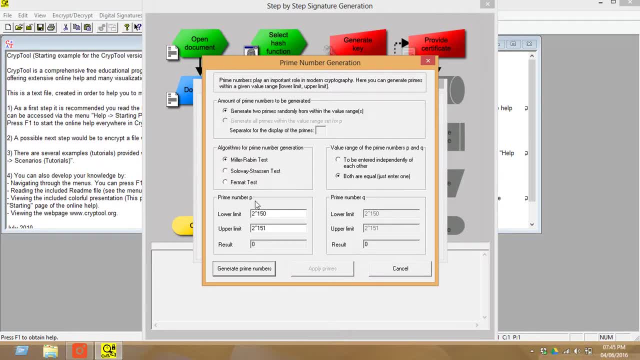 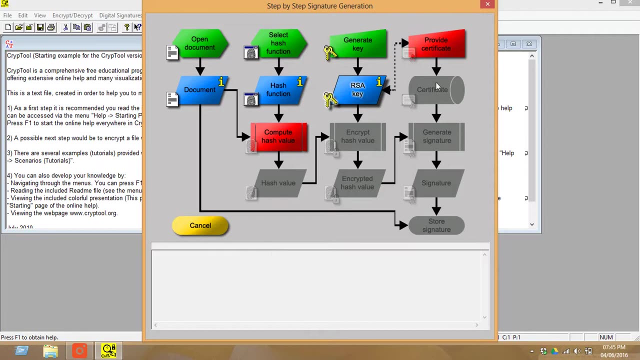 And the result is zero. This is for P, This is for Q, And click on generate prime numbers. Now you can see the results generated, two prime numbers and click on apply primes. Next you have to click store. Now click on this. provide certificate. In this you have to provide your name. 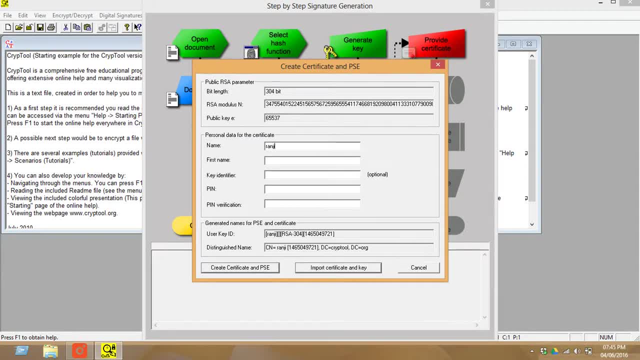 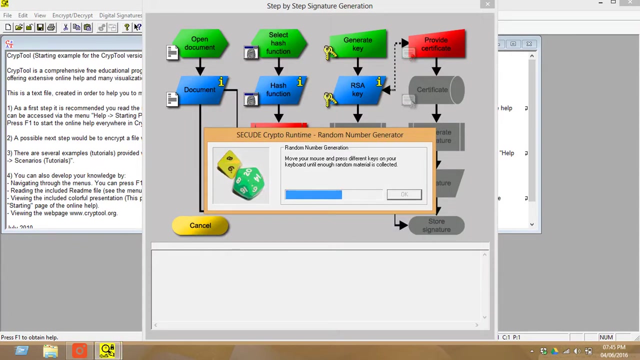 And this is the name. Next is the first name And this is the first name key identifier. that is optional, so tab anything and pin. I am typing crip tool and click on create certificate and PSE this the crypto runtime and it is created. now you can click on this. compute the hash value. hash value.